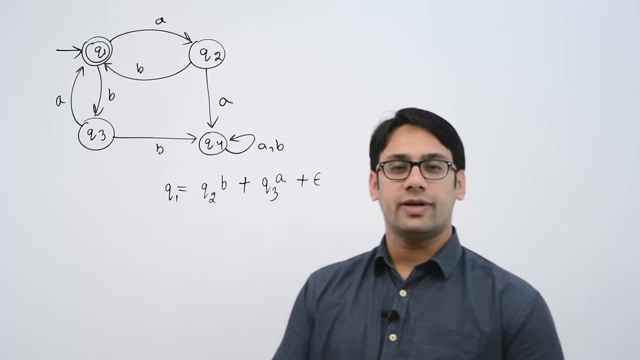 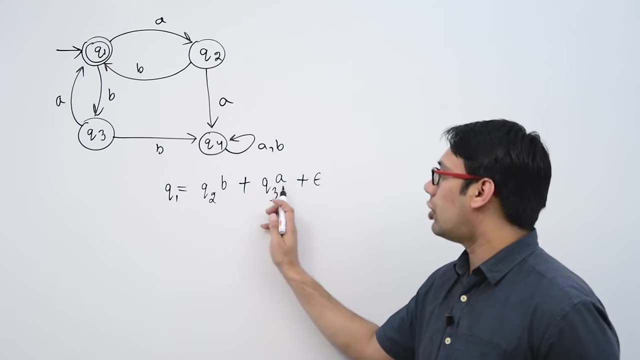 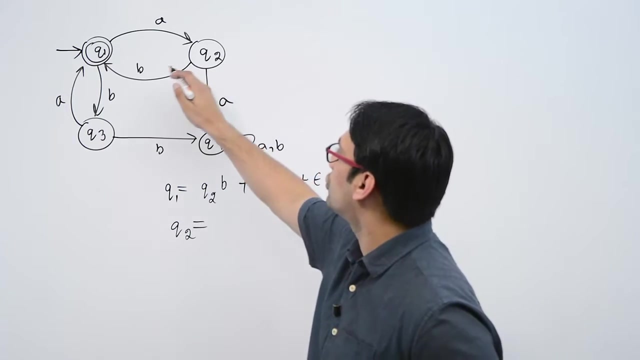 means you are at the start state, without just by seeing epsilon. you will be staying at the same state. So you can reach Q1 by seeing this, By seeing B at Q2 or A at Q3 or epsilon. If you are at Q2, how can you reach Q2?? To reach Q2, you have 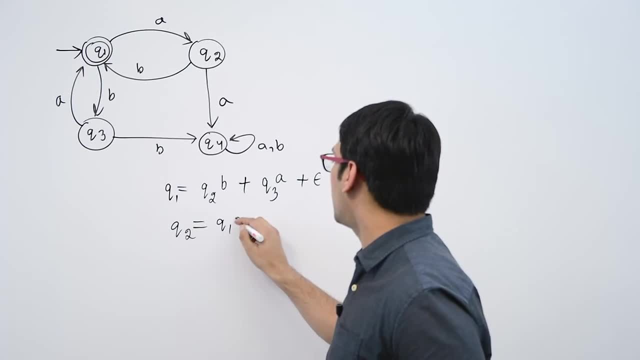 to see an A from Q1. that means if you have to see an A from Q1, otherwise there is no other method to reach to Q2.. If you want to reach to Q3, then you can only reach to Q3 only if you see B from Q1.. 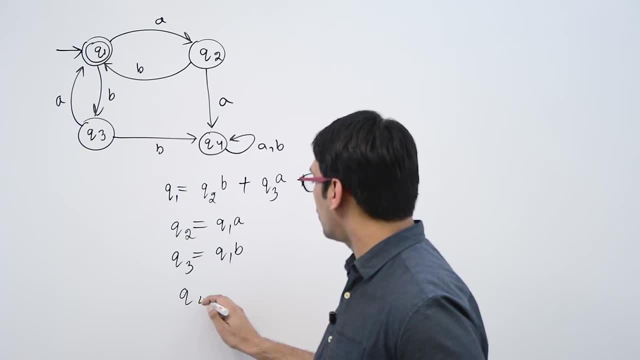 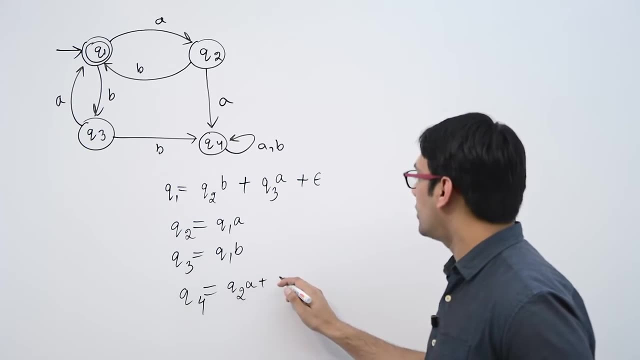 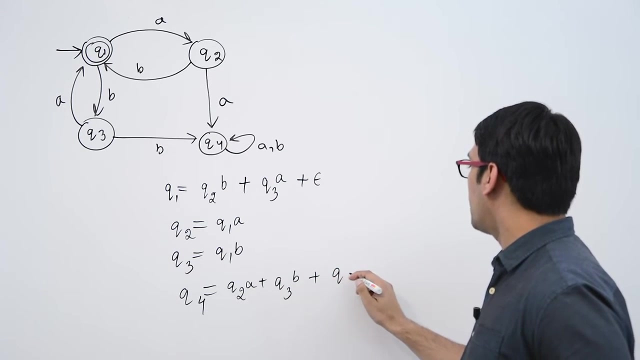 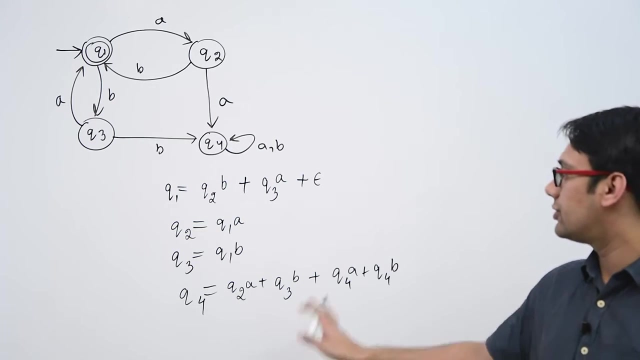 In the same way for Q4. you can only reach Q4 if you see an A on Q2, or you can see an B on Q3, or you can see an A at Q4 or B at Q4.. Ok, so this is the only method Here in this complete finite automata. 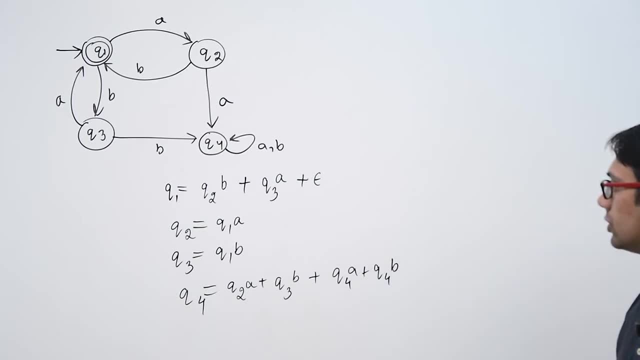 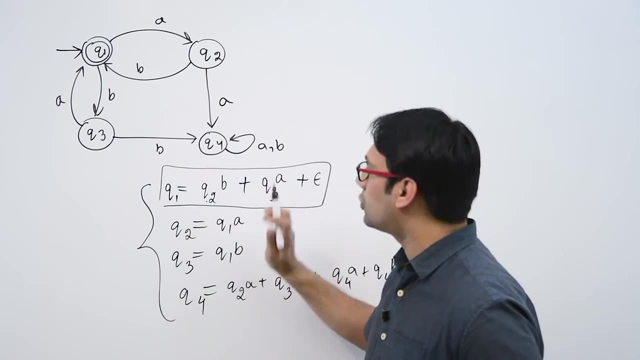 that is, Q1.. Q1 is the only final state. So here in all these expressions, if we can remove, if we can solve this expression by removing this Q2 and Q3 by the appropriate symbols, then we can get a regular expression Right. and we are going to extensively use the you know theorem, which is: 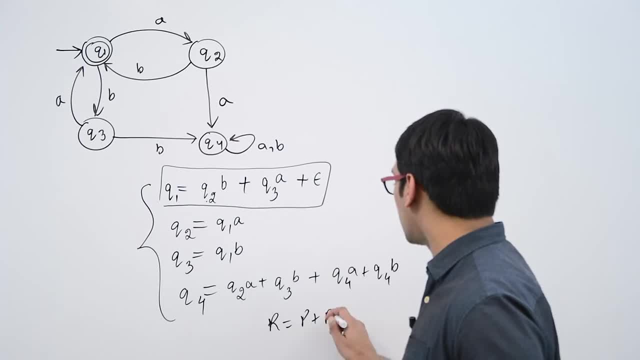 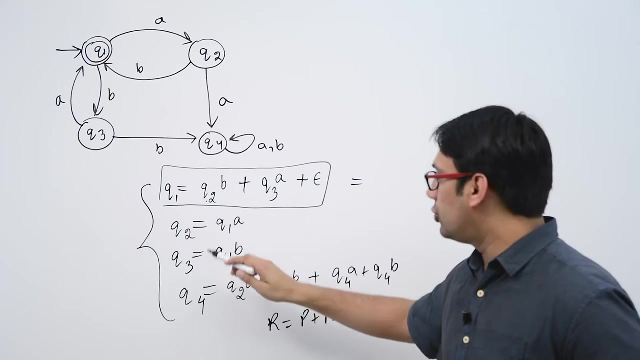 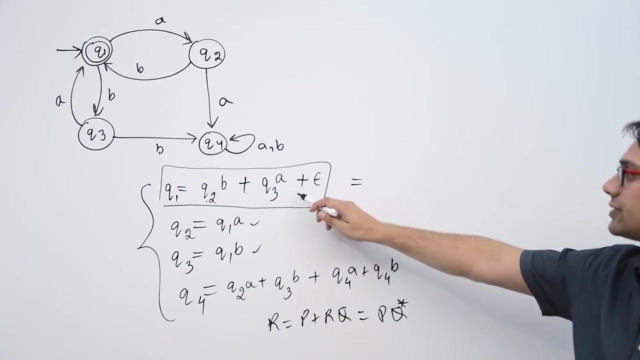 R is equal to P plus RQ. it can be written as PQ- star, which is the Ardennes method. Ok now, for example, here we have Q2 and we have Q3.. You can replace Q2 and Q3 by their exact values here, exactly because we have four expressions and we have to solve this expression we have to remove. 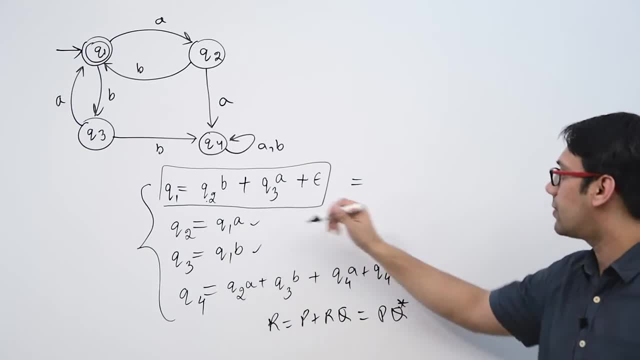 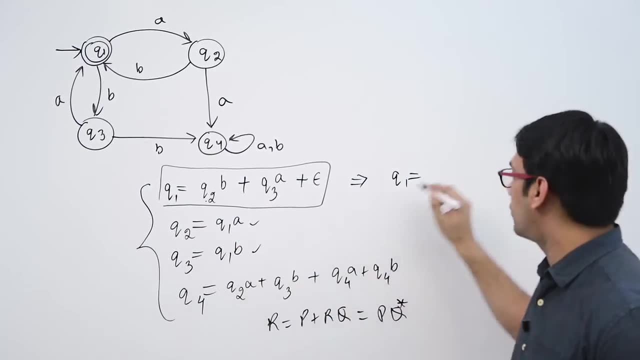 all the states, that all the present states. So the first expression can be written as: Q1 is equal to Q2B and the value of Q2 is Q1A. So Q1A dot B plus Q2B dot B. So this is the only way to solve this. 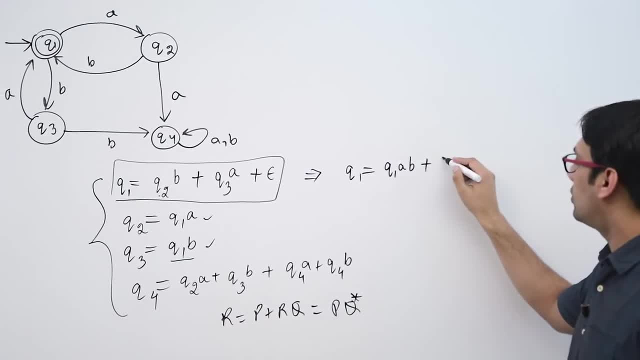 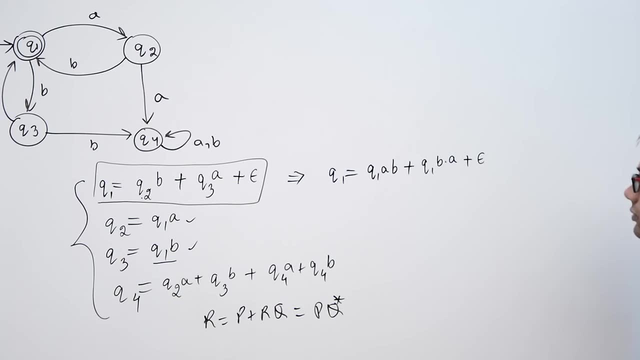 equation Q3 can be written as: Q1B plus Q1B, dot A plus epsilon. Ok, now this can be written as: Q1 is equal to epsilon plus take Q1 common, so it is Q1 dot AB plus BA. Now, if you compare it with the